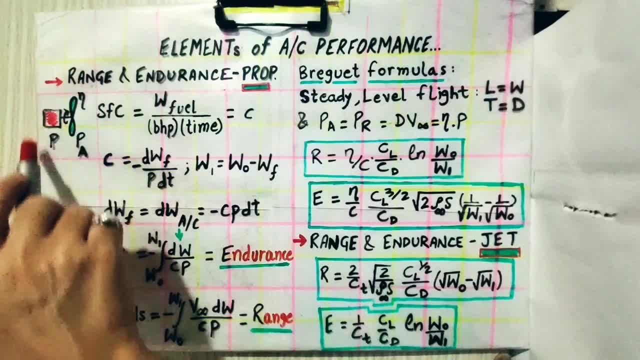 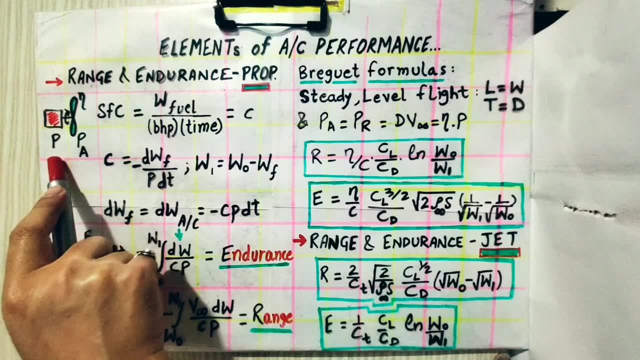 So here we have range and endurance for propeller airplane and this is the propeller engine. as you can see that the engine produces the piston engine specifically we are talking about. It is not a turboprop or turboshaft engine. It is a piston engine we are talking about and the shaft is rotating, the propeller and the power produced in the engine is the brake force. power p. 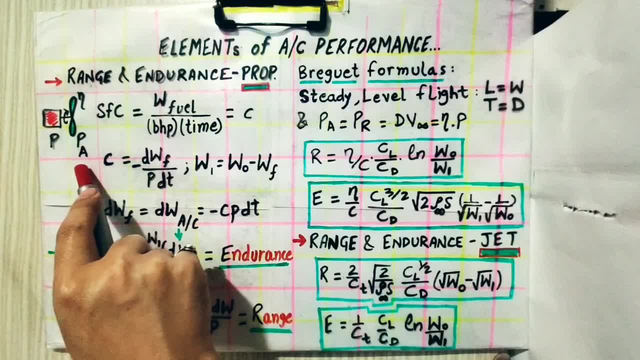 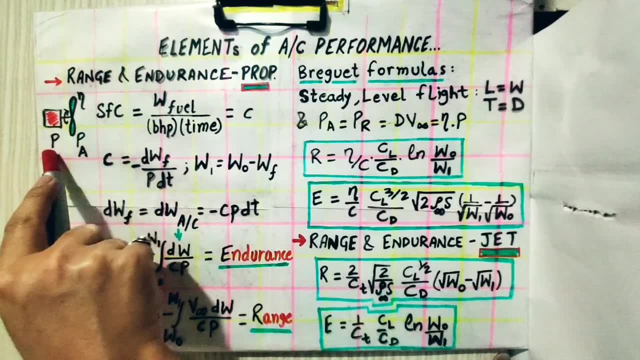 And the power available at the propeller end depends upon the efficiency of the propeller, amount of thrust it can generate and which brings us to the power available. that is equal to the eta times p. So the power available at the propeller end will be eta times p. 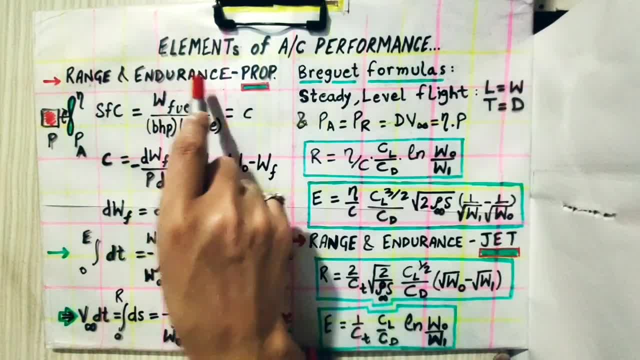 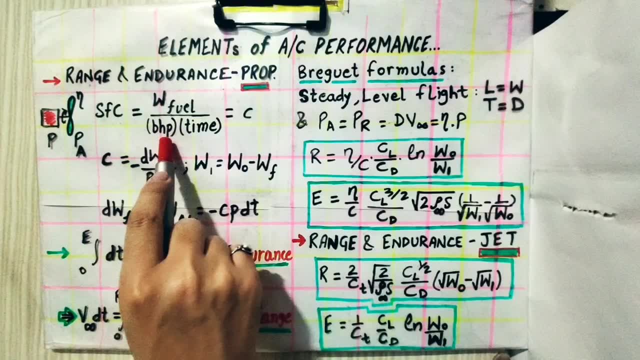 So in range and endurance we will see that power produced by the reciprocating engine is the brake force power, that is p, And the amount of fuel consumed in unit time to produce unit brake force power is the specific fuel consumption In propeller engine. we talk about the 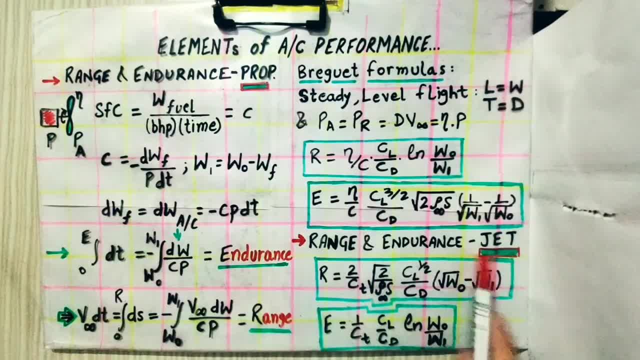 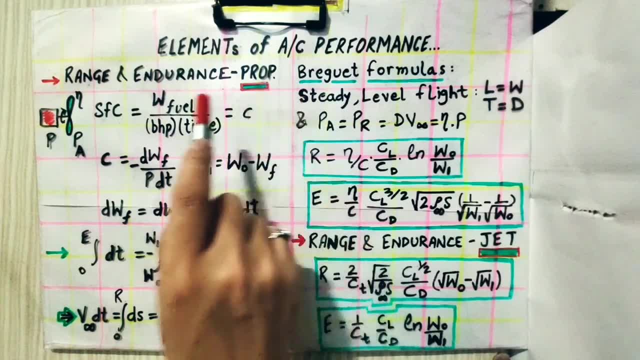 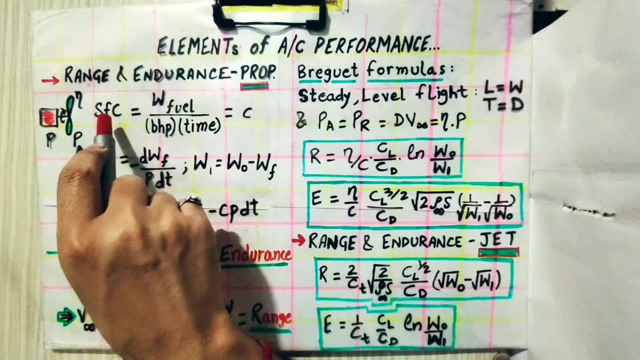 Power produced by the fuel consumption. but in jet engine we talk about the power fuel consumed to generate unit thrust for a unit time. The definition of specific fuel consumption just remain the same, only change the power parameter with thrust parameter in jet airplane. Okay, so let's first complete this power and it shows that amount of fuel consumed in unit time to produce unit power is given by c, which is specific fuel consumption. 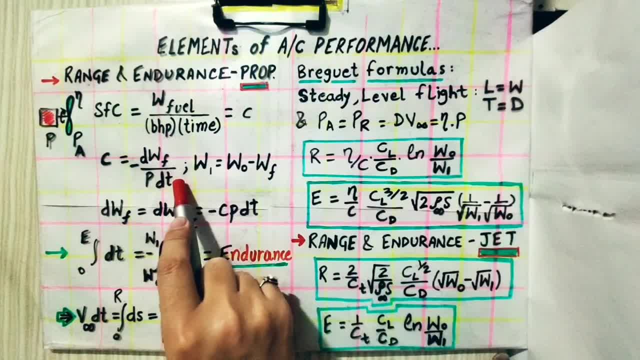 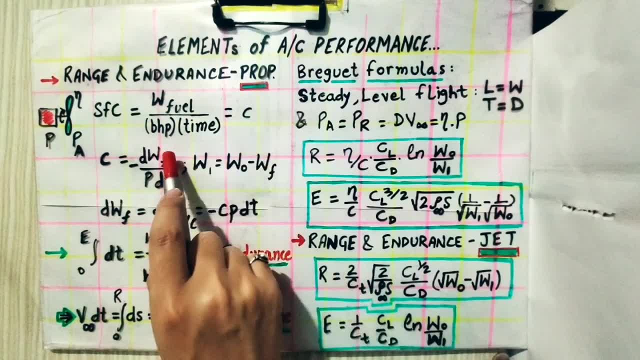 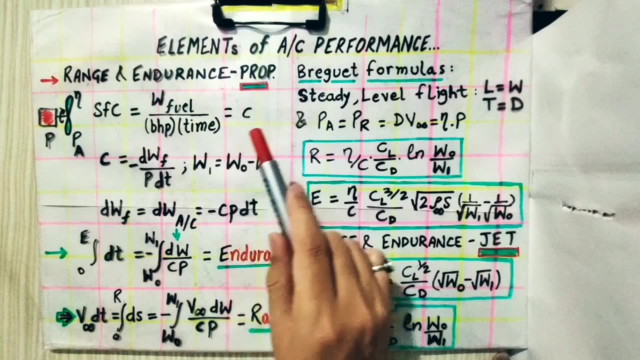 And the specific fuel consumption is written in this formula, Which shows that Minus dw of fuel. change in weight of fuel is decreasing because with time, as aircraft fly from one point to another, the fuel gets consumed and it will decrease, and the minus sign shows that it will decrease. the fuel will be consumed. 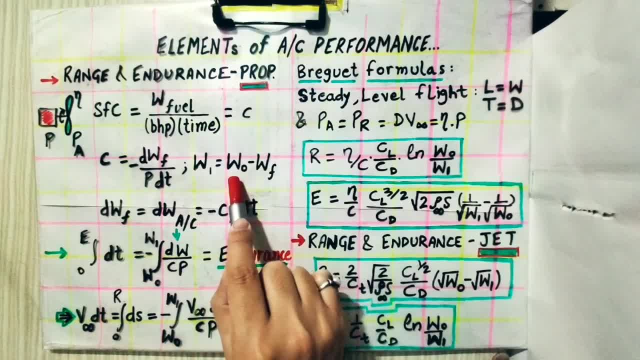 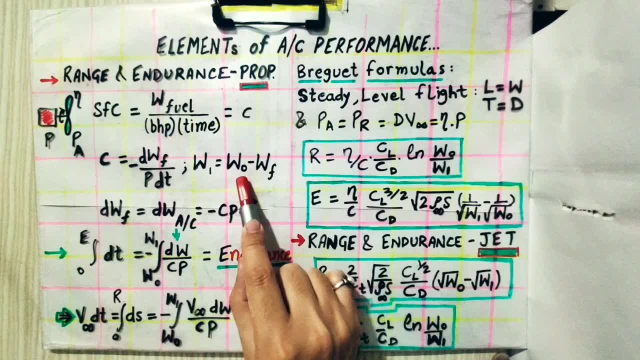 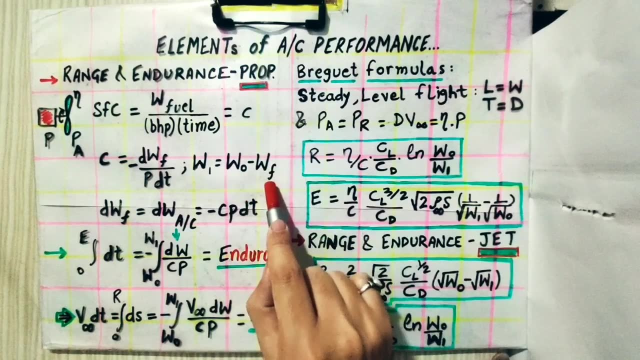 Okay, so let's say at initial time the weight of the aircraft, whole aircraft structure, payload or everything with fuel, its weight is w0 and when it reaches at a point its weight is w1, which is initial weight minus weight of the fuel. whole of the fuel is getting consumed. 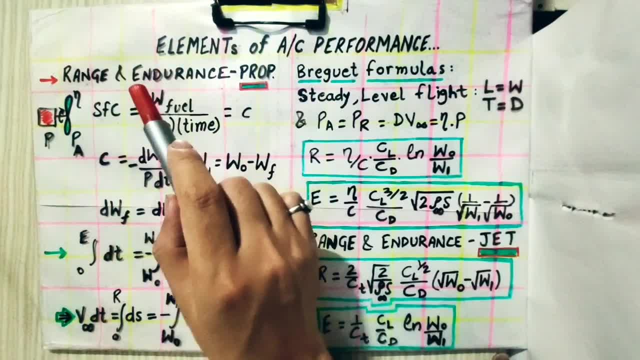 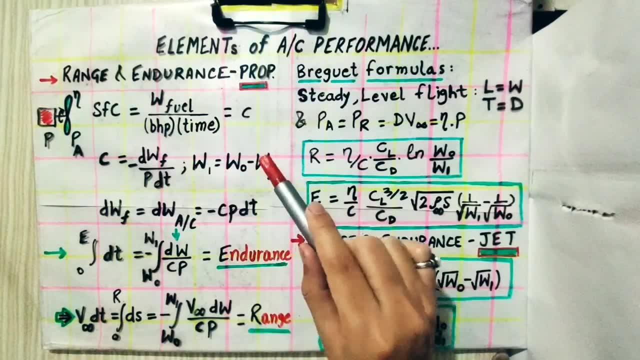 So now let's again revisit this definition of range and endurance. So the range for an airplane is actually the amount of distance it can travel for a given amount of fuel. Okay, the amount of distance we are talking about here for the aircraft is the distance with respect to the surface of earth. 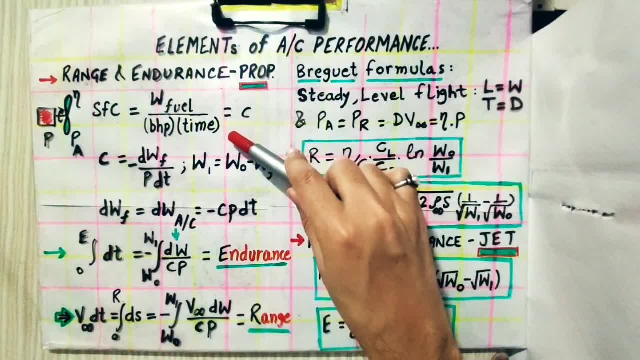 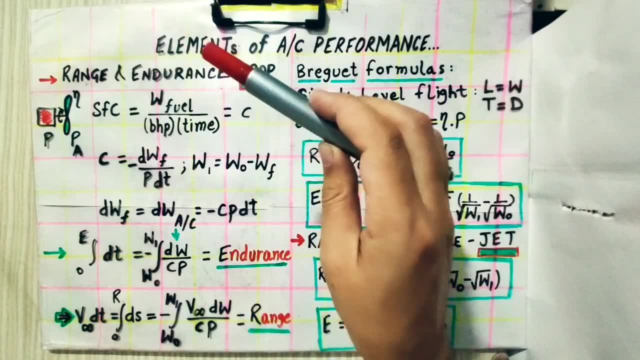 Okay, so the amount of distance it can travel in air, which is measured on the surface of earth, for a given tank of fuel is the range of an aircraft And the endurance is the amount of time it takes to cover the distance for a given amount of fuel. 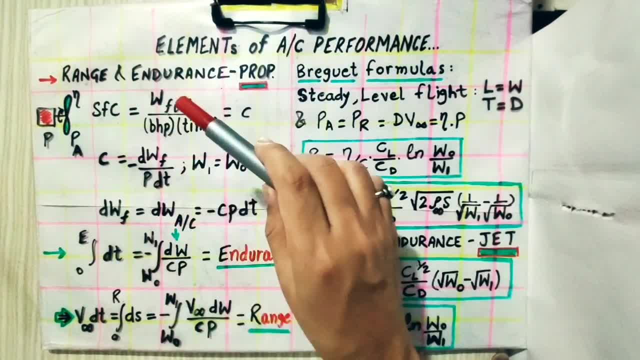 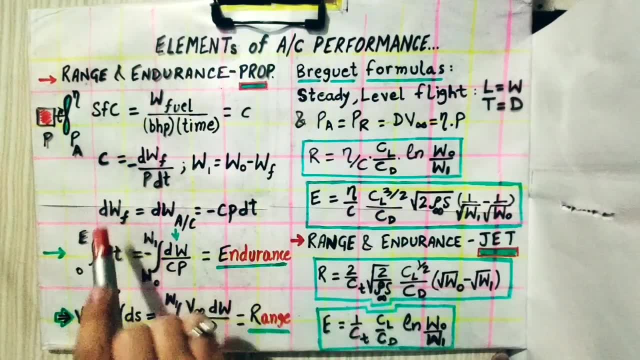 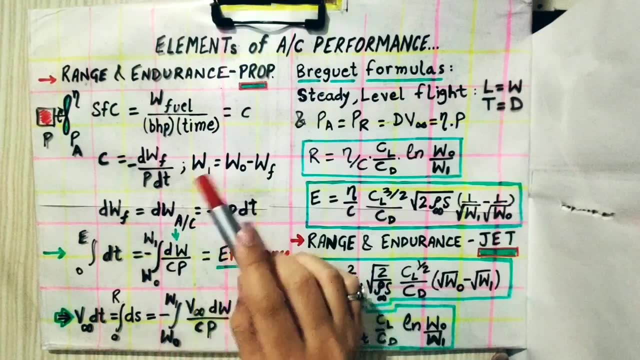 Okay, I will say: endurance is actually the amount of time the airplane can stay in the air for a given amount of fuel. Okay, so now let's complete it from here. we can say dwf is equals to dw of aircraft. that is, change in weight of fuel is equal to the change in weight of the aircraft, because the aircraft weight only changes because of the change in weight of fuel. 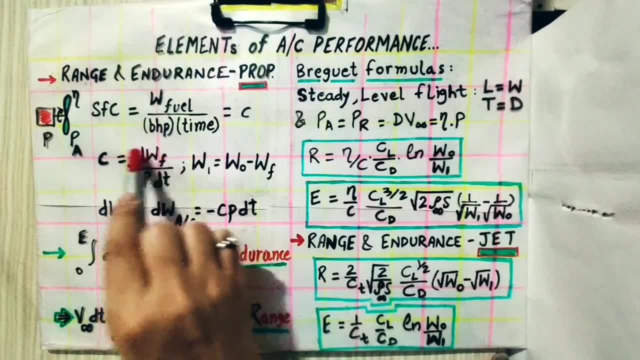 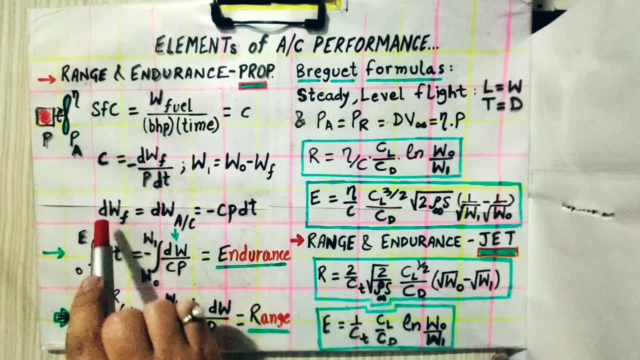 So the weight of the fuel when changes, the aircraft weight will change and it is equal to minus cp dt. Okay, so now here we can say, to compute the endurance, We brought minus cp dt. We brought minus cp dt Downwards of dw. 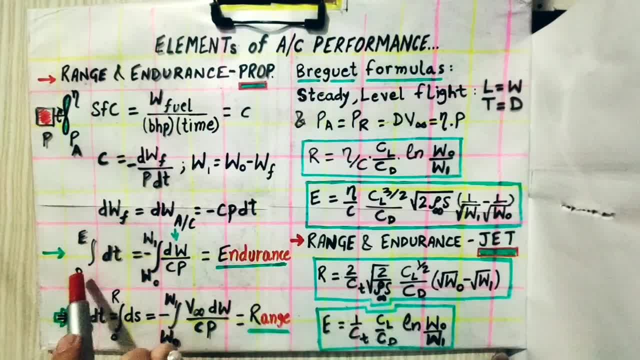 Okay, and from here we see that endurance e is just an integral from initial point zero to a time e. Okay for initial weight w naught of an aircraft to the final weight when the whole weight of the fuel gets consumed, w1. Okay, so integrating both sides with respective variables. 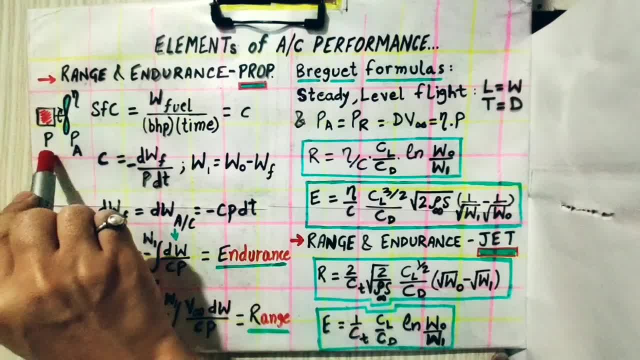 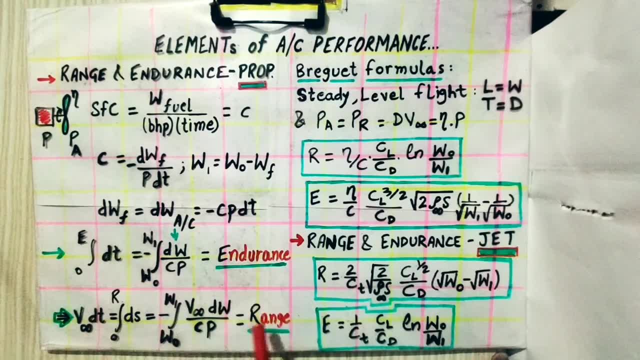 Okay, will give us the endurance of the airplane for a piston engine propeller driven aircraft, Okay. and similarly we can derive this range formula. We just need to multiply this time with velocity, because distance is equal to speed into time, And here we just need to multiply with the velocity of the aircraft. 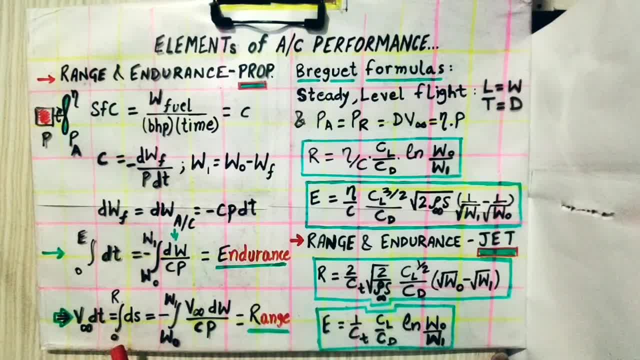 Which is v infinity, with which the aircraft is flying, and v infinity dt is equal to ds And from initial zero distance to r distance it can travel, and we just multiply this with v infinity and integrate it for same. w naught to w1, keeping minus sign outside. 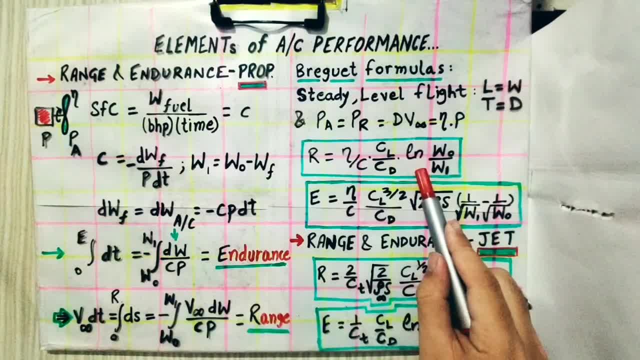 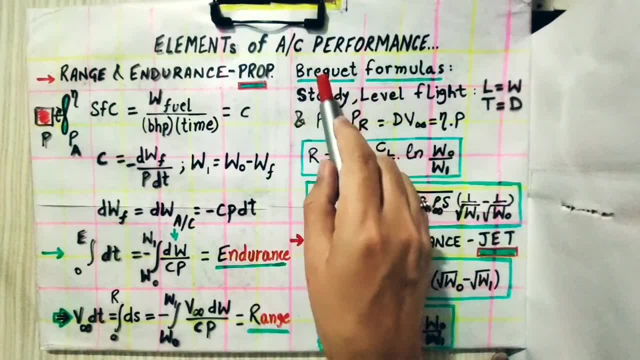 And this formula is further solved by using Burgett formula, by. it is a Burgett formula, Okay, and it might be pronounced in some other way, but I say a Burgett formula, Okay. so lift. for this Burgett formula, the lift is equal to weight and thrust is equal to drag. that is here. 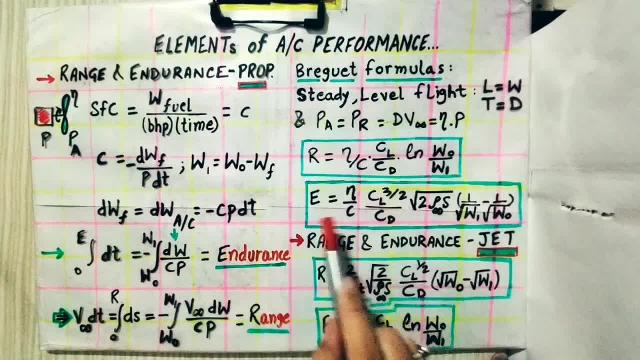 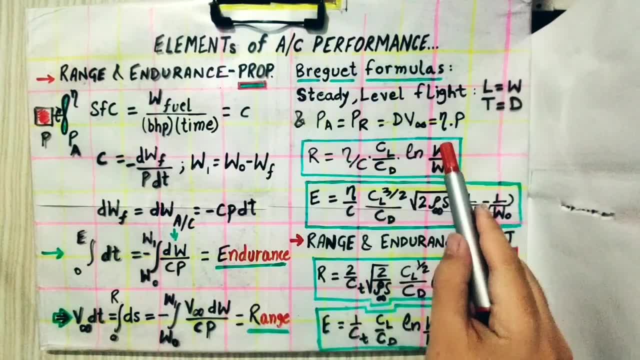 We are considering A steady level flight, to derive the range and endurance formula, a complete formula, a closed form solution. We can say that will give us the amount of range if we know the given parameters for an aircraft. Okay, so we substituted value of lift and drag over here. 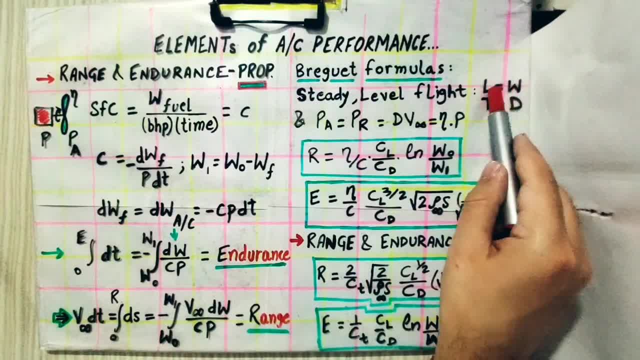 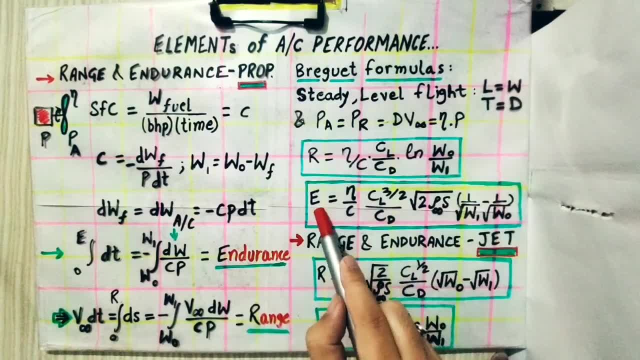 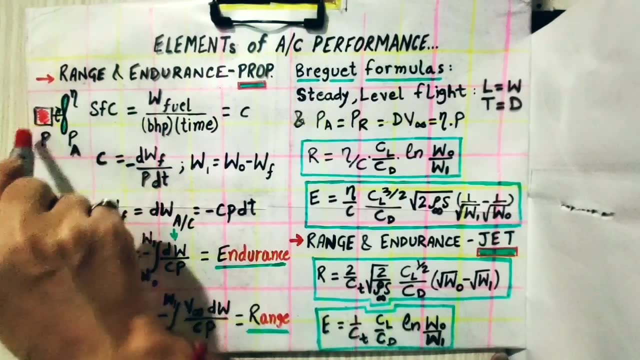 Okay when this is integrated and upon substituting value of lift, thrust or drag over here and substituting value of this power p, because the amount of range or endurance for an piston engine airplane who is driven by propeller Will depend upon that amount of power that is brake horsepower produce by consuming the amount of fuel in the piston engine. 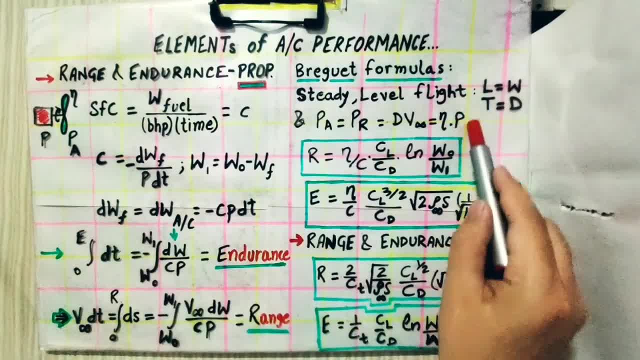 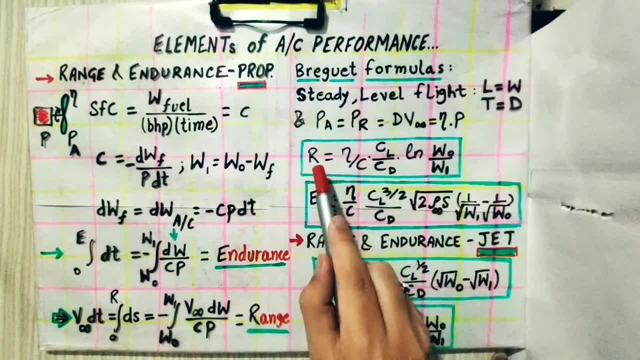 It does not depend on the power available at the propeller engine. okay, so that is that why we are using this p over here. okay, In this formula, not power available. This is brake hose power and upon solving we will get the range equals to eta by c multiplied by c, l by c, d multiplied by ln. 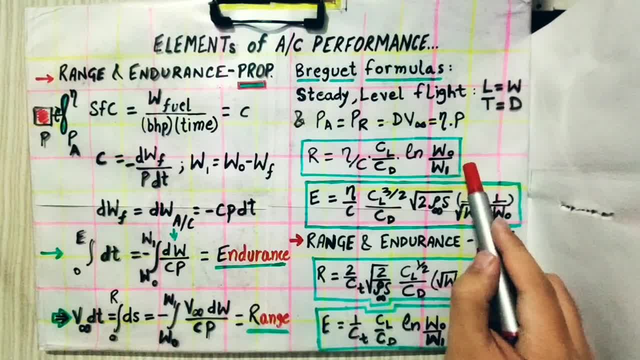 That is natural log of w, not by w. 1 initial and final weight and endurance is eta by c, multiplied by c, l, raised to power 3 by 2 by c d, under OM earth, which is upon this fundamental function that we have. enterance is eta over this. this has the Medicine range, so this always intensively individually트� metadata. another similar nữa here as used and is the intrinsic unit, initial and final weight and the predators. basically, no, gonna use the derivative and not static. 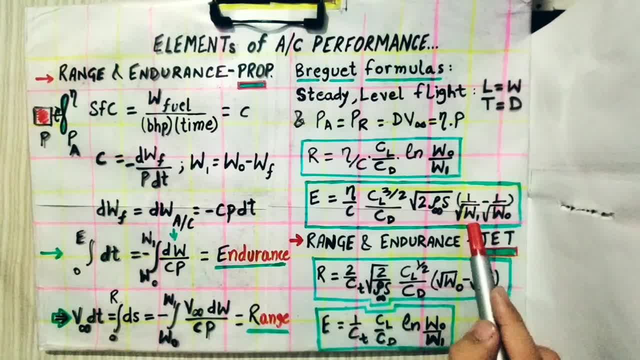 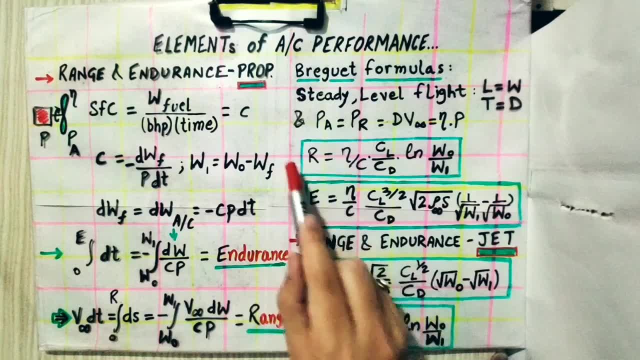 root of 2, rho infinity s multiplied by 1 by under root w1 minus 1 by under root w0. and if you see or compare these formulas, that you will see that range does not depend upon the density, whereas endurance depends upon the density. or say, as the aircraft, a propeller driven aircraft with 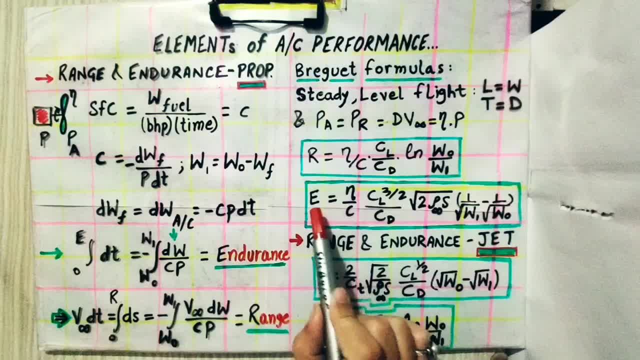 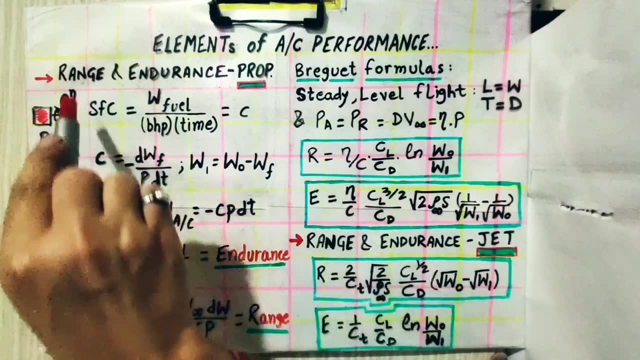 reciprocating engine flies at sea level. where density is maximum, endurance will be maximum and range does not depend upon the altitude at which the airplanes are propeller driven. airplane is flying okay with a piston engine and other points remain the same for both these except one another: that range and endurance will increase when efficiency of propeller is maximum. 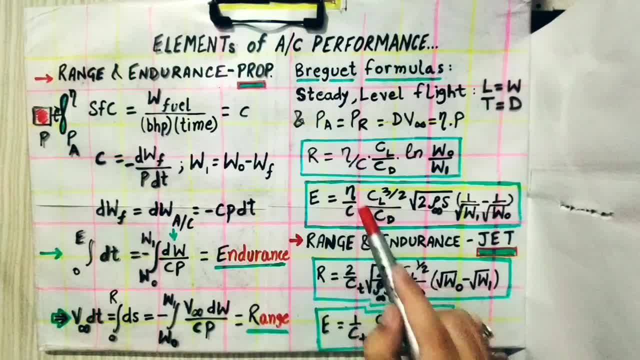 or will be high, and the fuel consumption should be the lowest, then range and endurance will be high. also, the initial weight, that is, w0, of the aircraft should be high, or say the weight of fuel should be high, okay, which is why the range or endurance will be maximum. and lastly, for the range to be 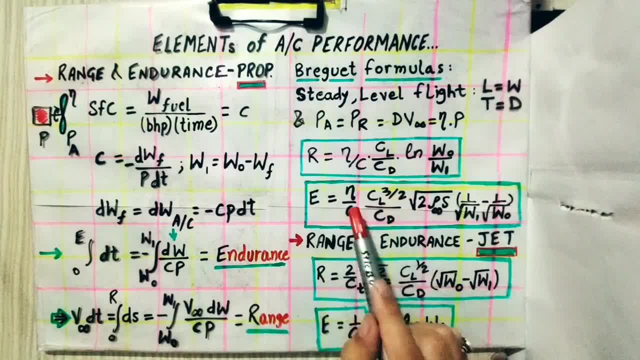 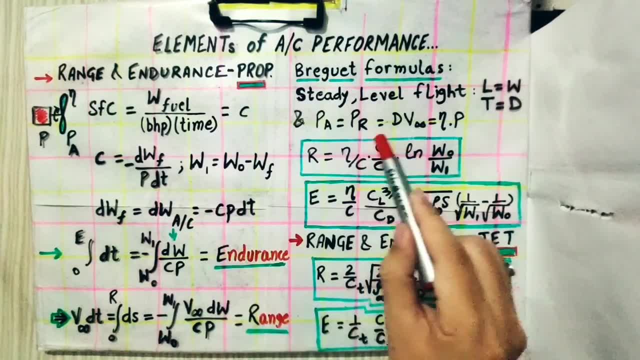 maximum cl by cd should be maximum, but for endurance, cl raised about 3 by 2 divided by cd should be maximum. okay, we have done these while doing our power required and thrust required and at that time we have seen these are design points for an aircraft performance and we will. 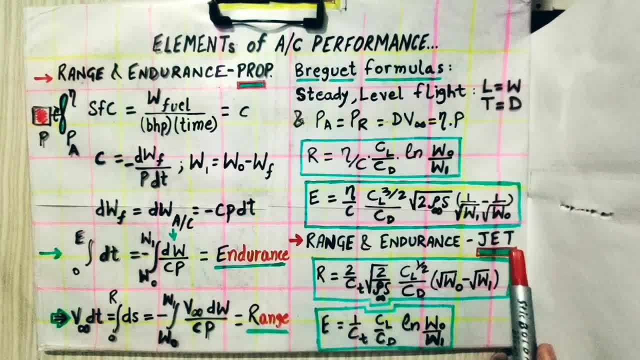 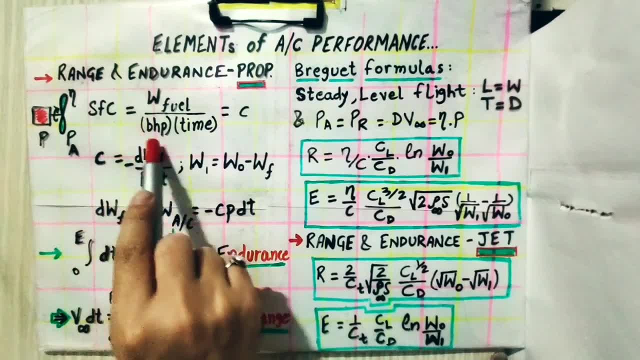 again revisit this in the next lecture. and now, moving on to the range and endurance for a jet engine airplane, we have seen that this specific fuel consumption is just different in this power term, that because the amount of fuel consumed here in a piston engine is generating power to 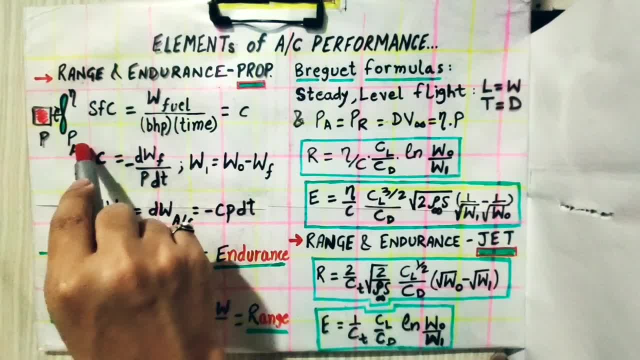 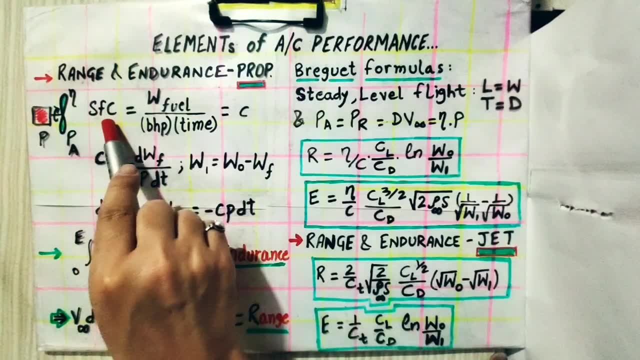 rotate the shaft so that it can deliver the power to this propeller. that should be the fuel. fly an aircraft with the available power at this propeller. but for an jet engine airplane, the amount of fuel consumed depends upon the amount of thrust it can generate at the end of. 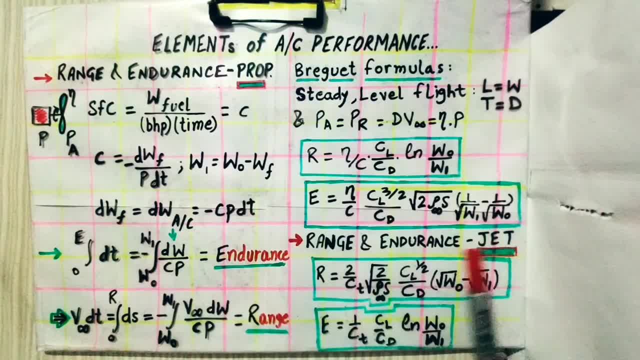 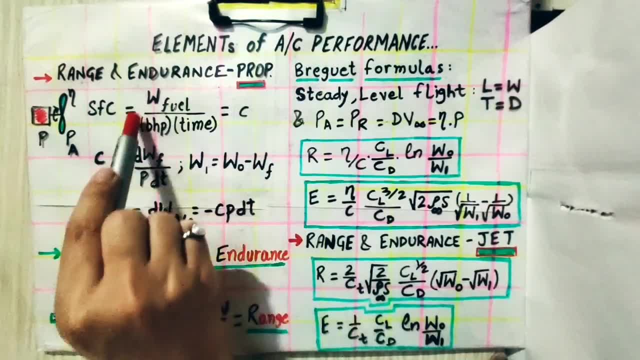 the nozzle of the aircraft, okay, or at the end of the jet airplane. so, which is why the specific fuel consumption for jet engine will give us the formula, that is, weight of fuel consumed to produce unit thrust for a unit time. okay, here bhp will be reduced by thrust, which is equal to drag, and 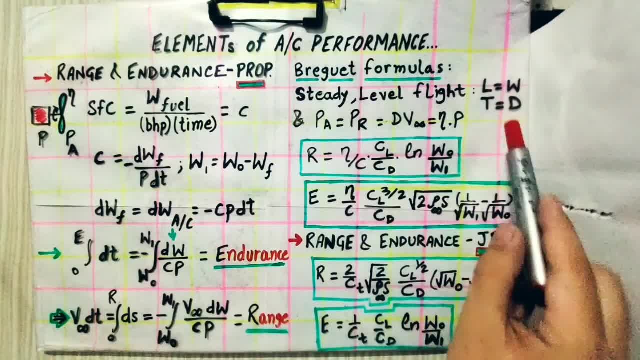 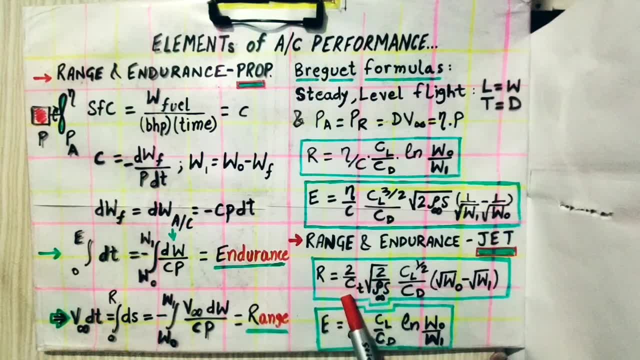 then the range and endurance formula for steady level flight will be derived for these parameters and we can see that range is equal to 2 by c or it is. here it is specific: fuel consumption is c and here ct. and please note the weight which we are talking about here: w naught initial weight. 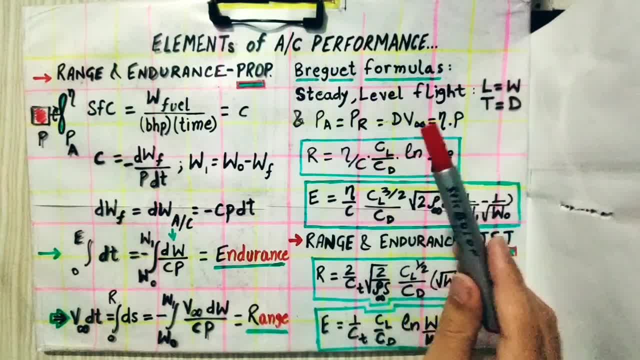 everywhere. we are talking about initial weight. w naught is an instantaneous weight at that moment. what is the weight of an airplane? okay, at an instant we are talking about, and as the time goes, the weight of the aircraft keeps increasing because the fuel is getting consumed, so the range of jet 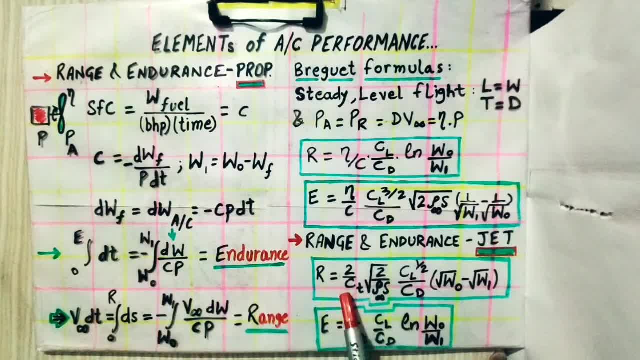 engine aircraft is given by 2 by c, or say ct, which is specific fuel consumption, for which is again range, is equal to 2 by ct. under root, 2 divided by ct, which is equal to 2 by ct, which is equal to 2 by ct. 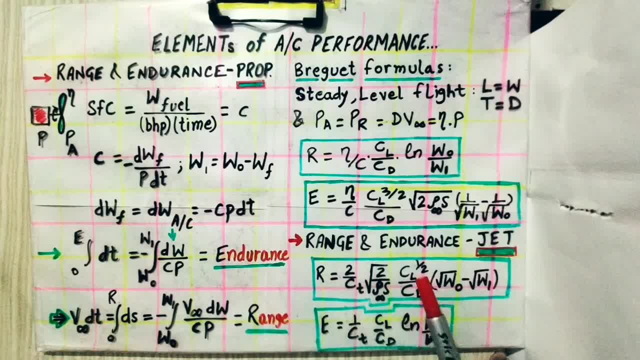 rho times s or rho infinity times s s is the platform area we know from aerodynamics. okay, and it is multiplied by cl, raised to power 1 by 2, divided by cd, multiplied by under root w0 minus under root w1, this is range for a jet engine airplane and the endurance is given by e equals. 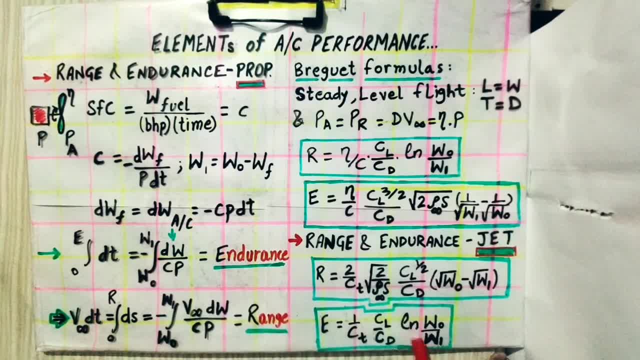 1 by ct, multiplied by cl by cd, multiplied by natural log ln of w0 by w1. so here also we will see that both these- fuel consumption, for jet engine as well, should be the minimum for range and endurance, and initial weight should also be high, or say it should be maximum, or when it will. 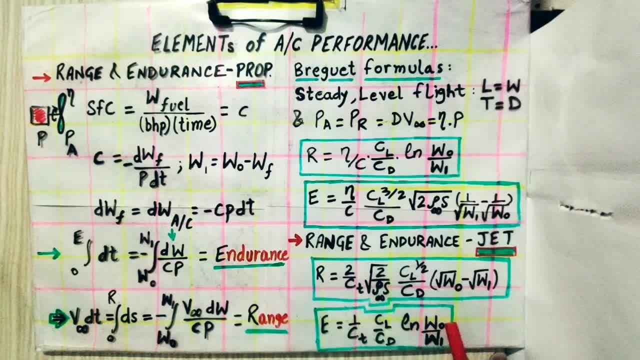 be maximum when the amount of fuel will be maximum. okay, initial weight will be maximum when the amount of fuel will be maximum. or now the other parameter that differentiates range and endurance. over here, for a jet engine, the range depends upon the altitude at which it is flying. the higher the 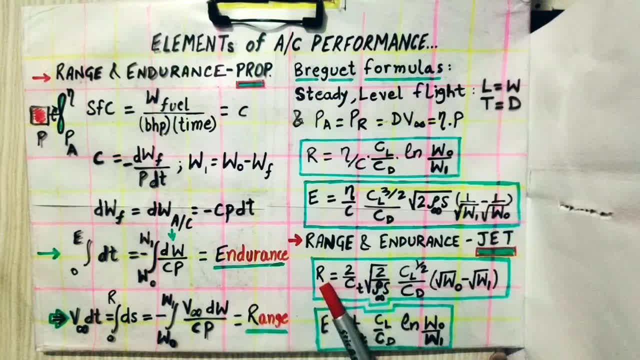 altitude, the higher the range. so- but a caution should be taken here- that higher the altitude it may be outer atmosphere where there is no atmosphere, outer space actually, where there is no atmosphere. so there is no point of jet airplane that will be flying, so we should stick to this. 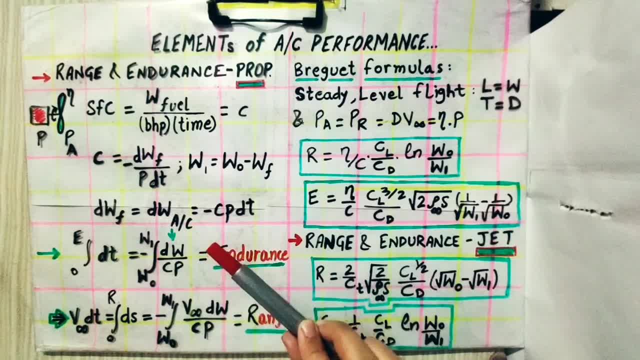 that range is the worst when it is flying at sea level and it increases as it goes at higher altitude and endurance does not depend upon the altitude at which the jet aircraft is flying. and another parameter at which range depends is cl is about 1 by 2 divided by cd. these cl and cd. 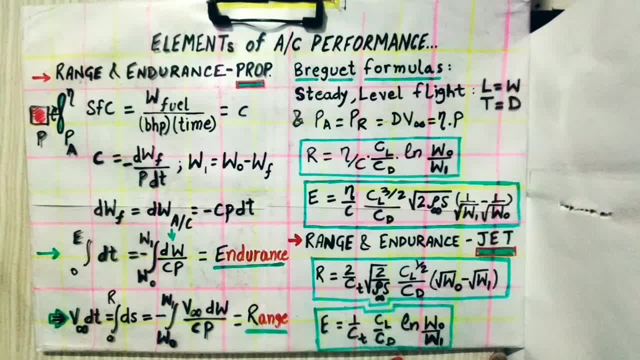 ratios in these formulas are all aircraft performance or aircraft design parameters, which is why they are important. okay, and here we see that endurance is dependent upon cl by cd ratio and we know that cl by cd is just required minimum. okay, cl by cd will be maximum at thrust required minimum. and lastly, we can see a little similarity. 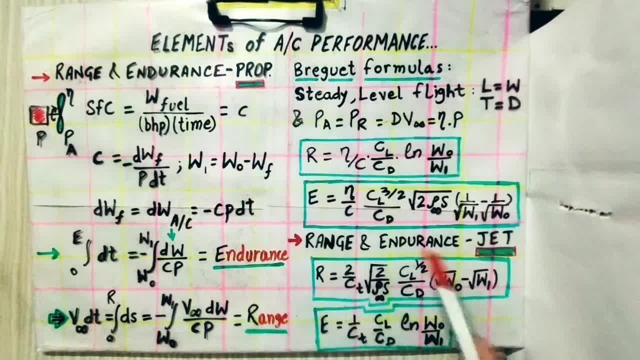 and opposite formulas in these propeller and jet engine. that range formula is quite similar to the endurance formula of propeller, for the range formula of jet is similar to endurance formula of propeller and endurance formula of jet is similar to range formula of propeller. so keep this in mind. we will continue next lecture. thank you. 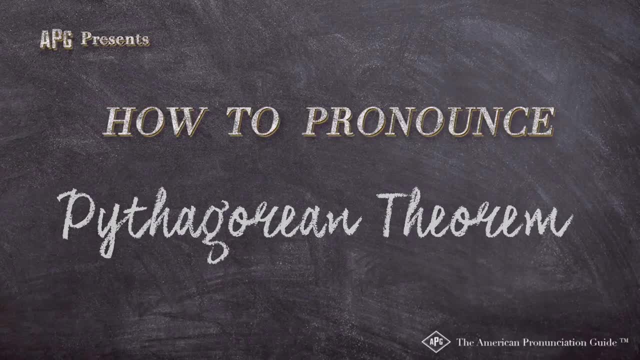 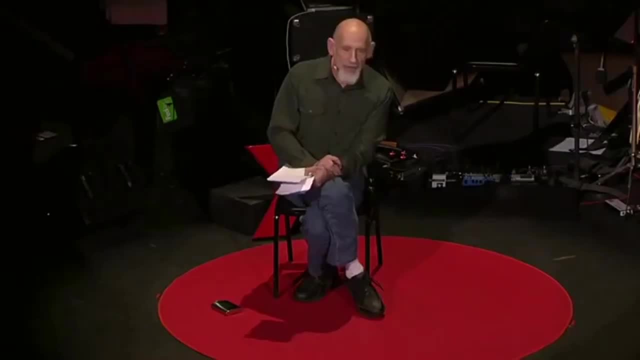 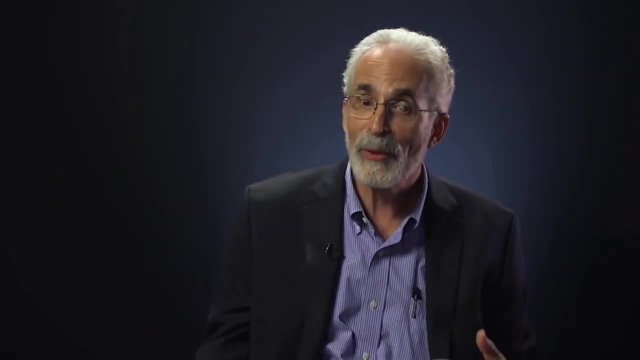 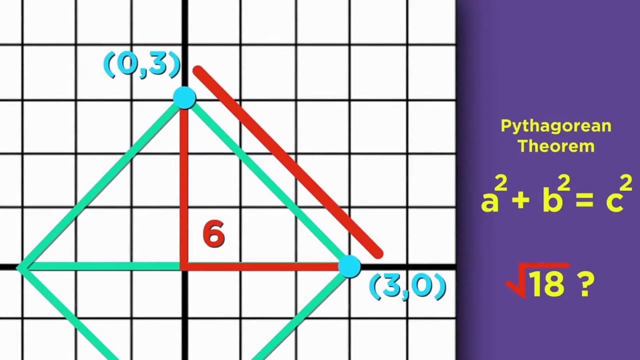 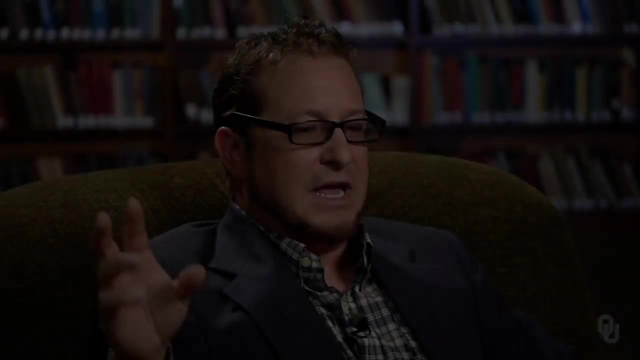 The American Pronunciation Guide Presents ''How to Pronounce Pythagorean Theorem''. He even taught me the Pythagorean theorem. They haven't learned the Pythagorean theorem But your intuition. and the Pythagorean theorem is that the slave boy is able to state and to articulate the Pythagorean theorem. 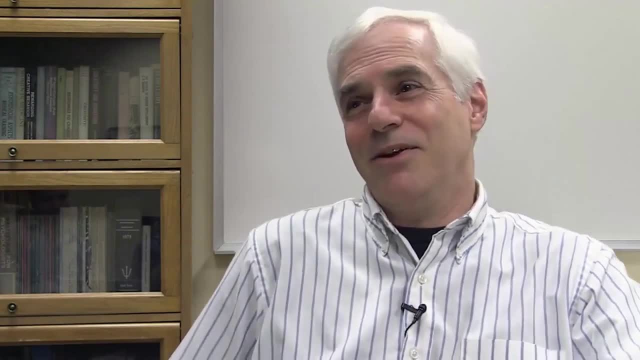 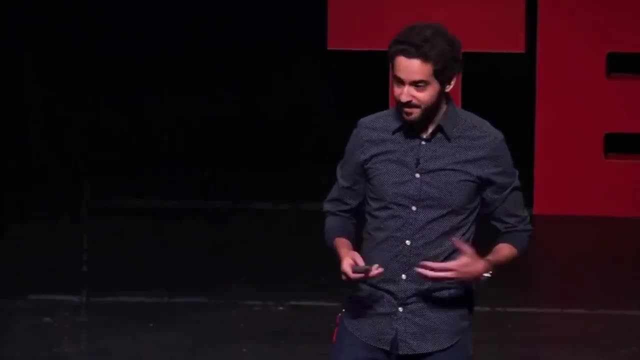 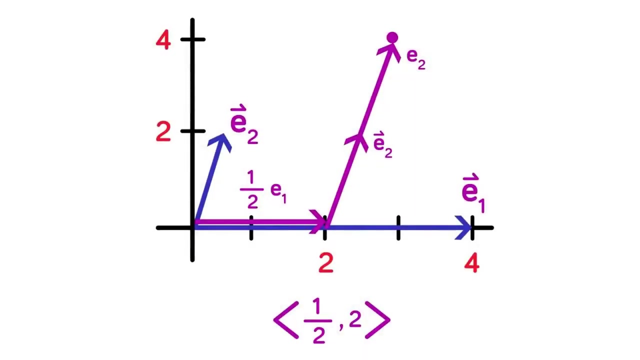 the Pythagorean theorem. the Pythagorean theorem. Now, if you want to find the distance, the Pythagorean theorem will not work.